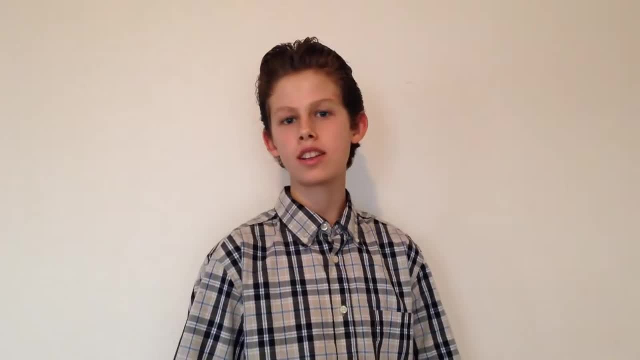 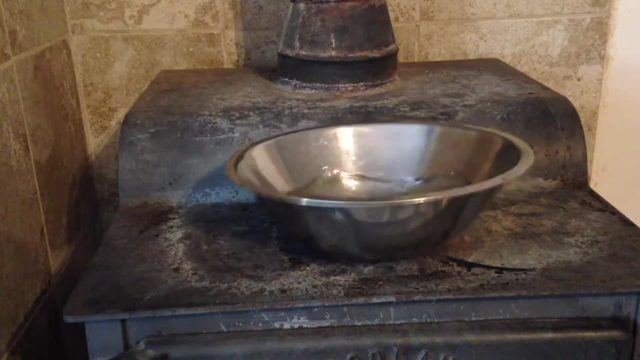 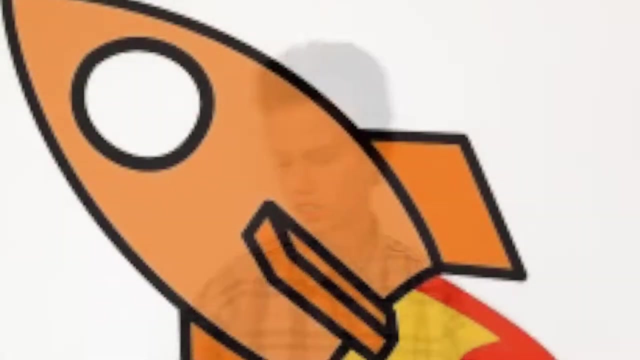 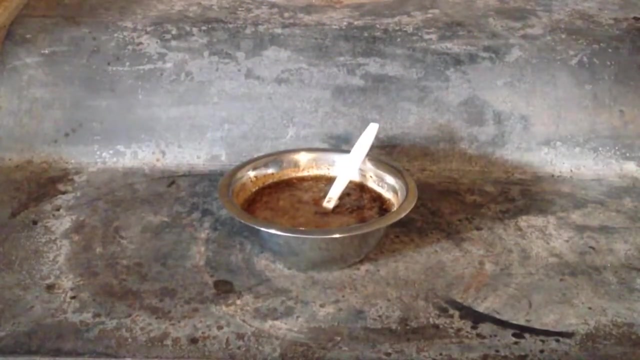 Hello, this is Jonathan with Super Science, and it's time to discover why this happens. So, guys, this is really weird. We need to get to the bottom of this. You're watching Super Science. I discovered this watching my dad put his bowl on the stove. 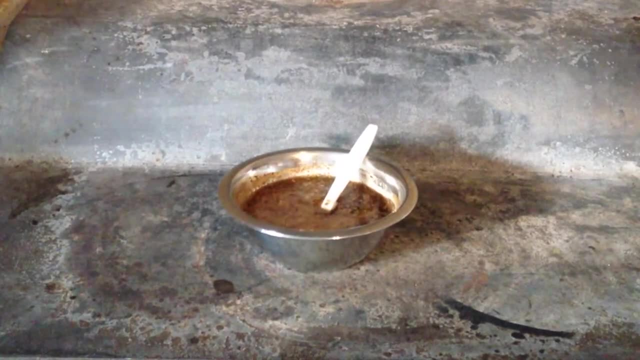 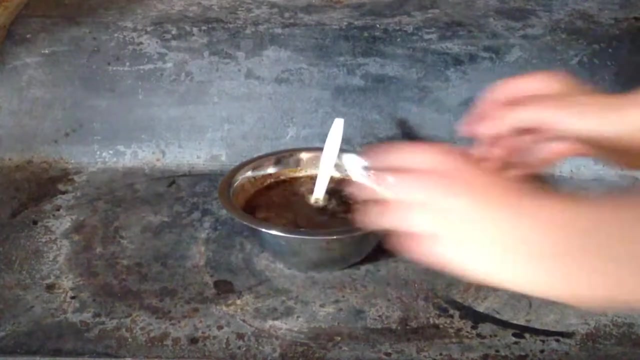 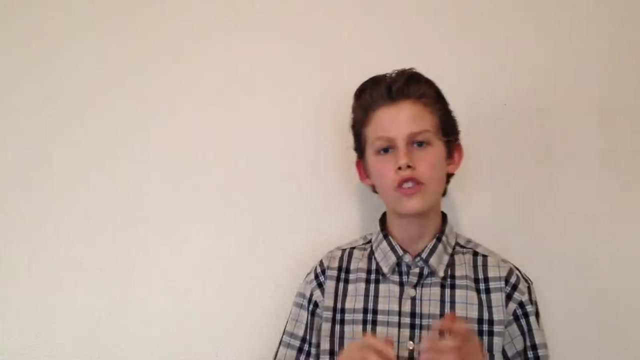 so I decided to share with you the science behind how this works. So, watching as I stop it, it starts up again. This is really weird folks. Why is this happening? So in order for this to be good science, it needs to be verifiable, repeatable. 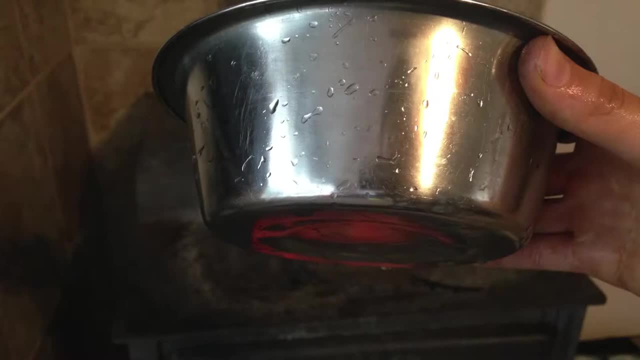 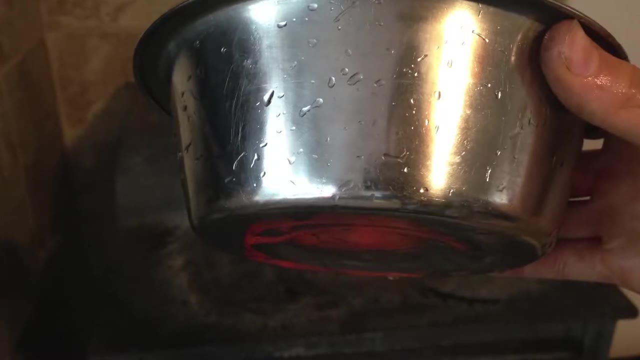 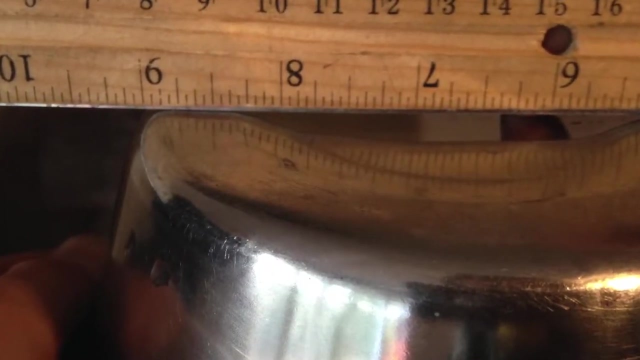 and it has to make sense. So I got another bowl here, But this one got a slightly different make to it. It's bigger and it got a flat bottom. So there should be no way that this can have the same effect as the other one. Let's see. 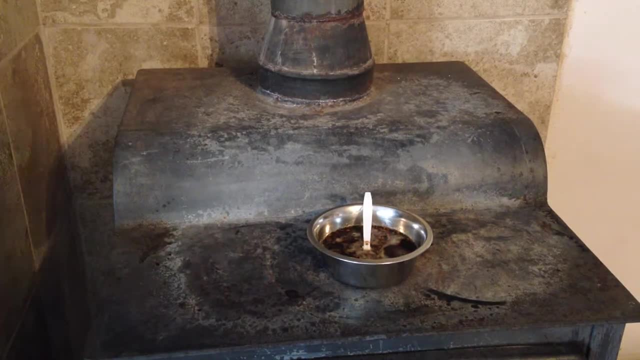 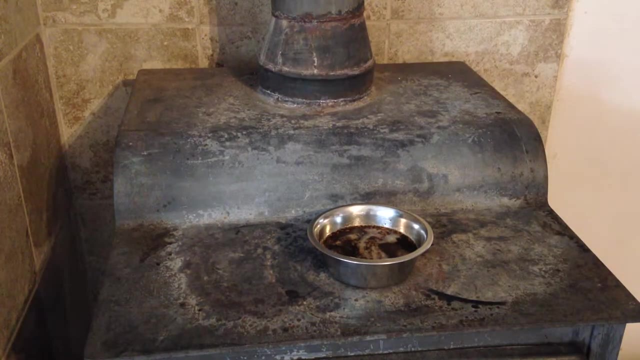 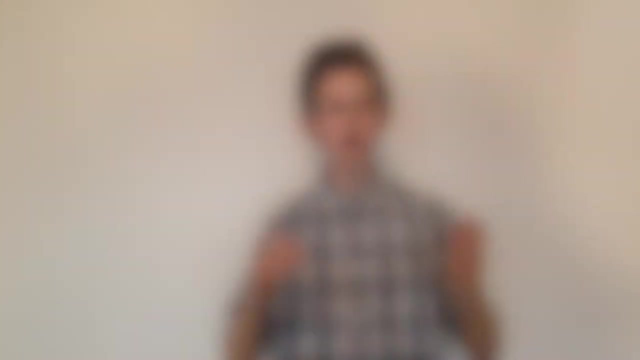 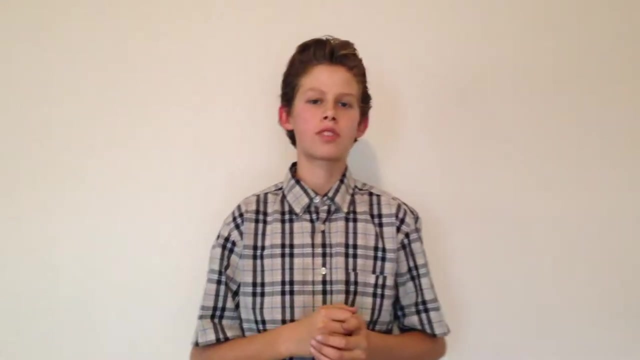 I'm gonna have to take this spoon out so it doesn't melt, But the difference is that they're not the same. Let's just try again. Let's wait to see if it still happens. Okay, This is neat and all, But we also know that bigger's better, So let's try something else. 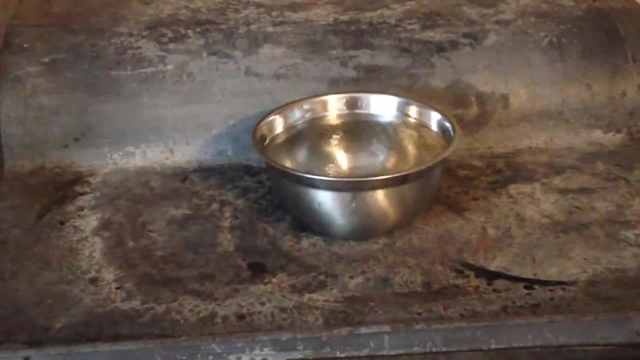 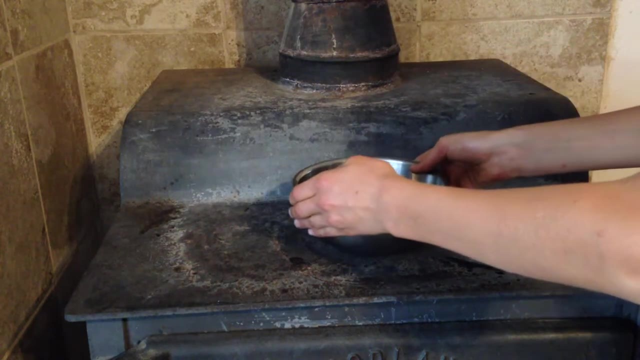 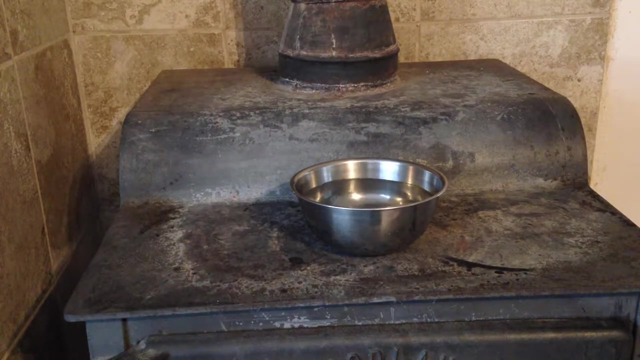 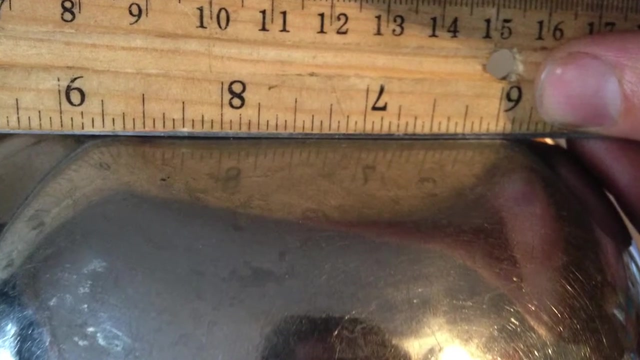 That was cool. let's try this bowl now. As we can see, it is not moving at all. What is going on? Maybe it has something to do with the structure of this bowl. The bottom of this bowl is flat, just like the other bowls. that wouldn't work. 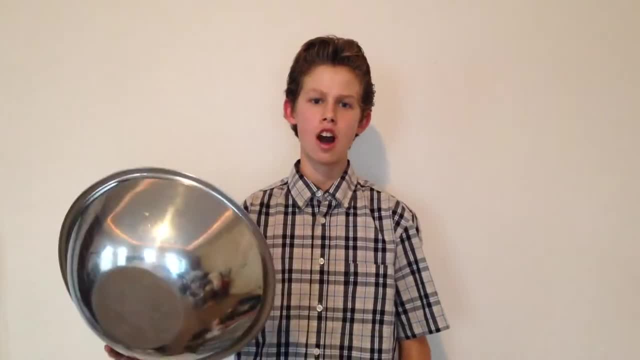 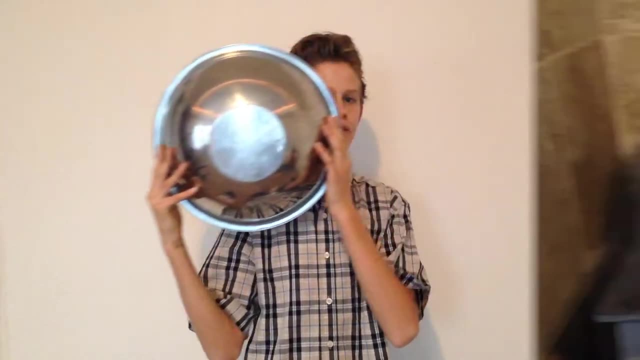 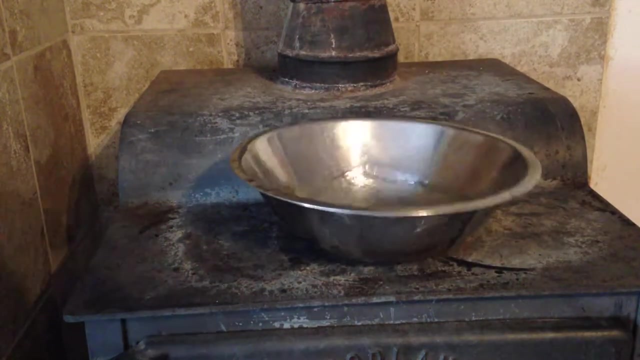 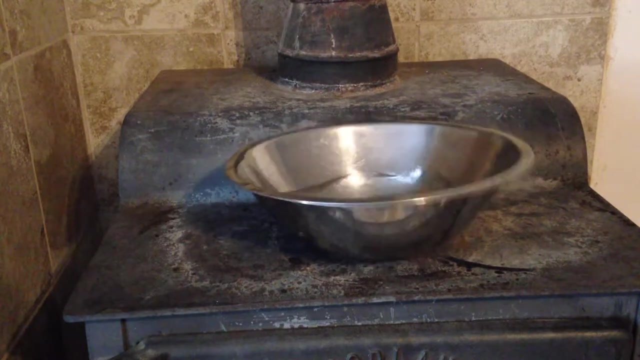 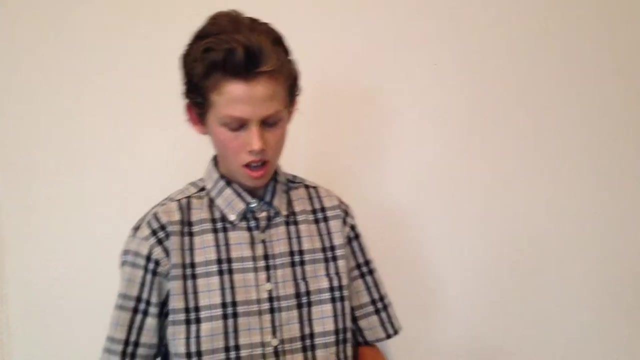 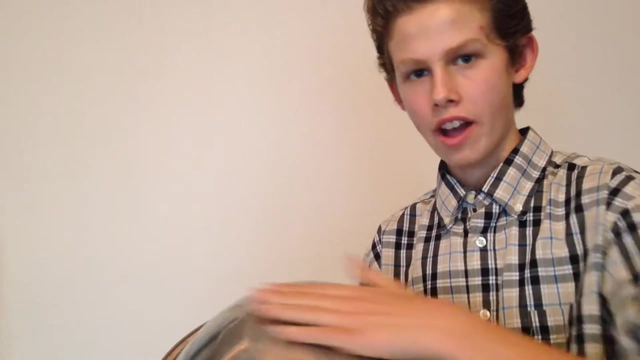 But I just happen to have the granddaddy of all bowls. Alright, let's try it. It's working And this is what it sounds like in reverse. But why does this happen? If you look closely on the bottom of the bowl, it's rounded. 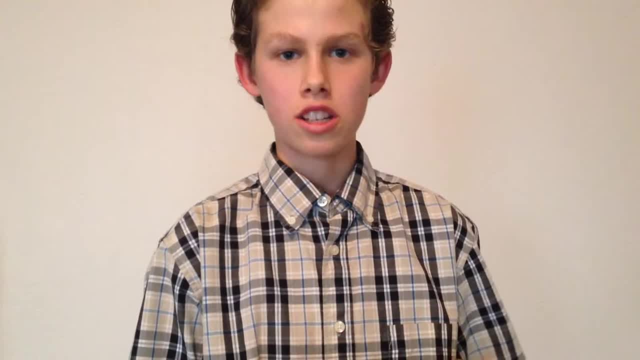 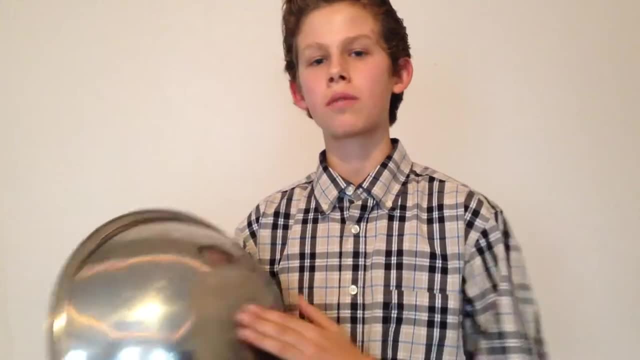 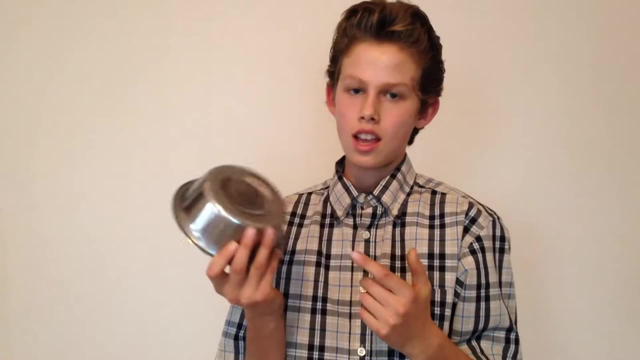 On all the bowls that wouldn't work, The ones that wobbled and danced on the stove, They all had this rounded bottom to it. So it must be something to do with the rounded bottom, because when you have one of these with a flat bottom, there's no way this can happen. 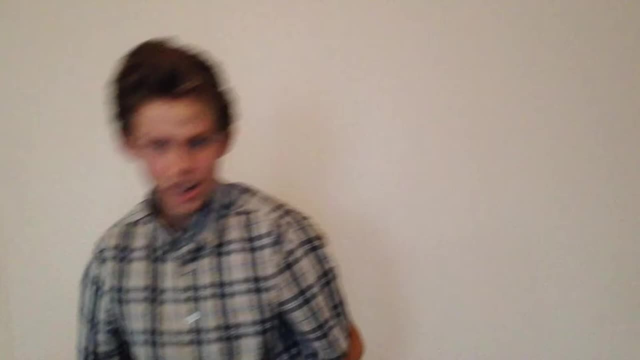 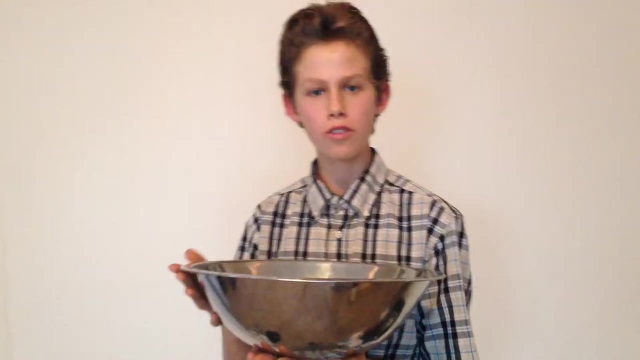 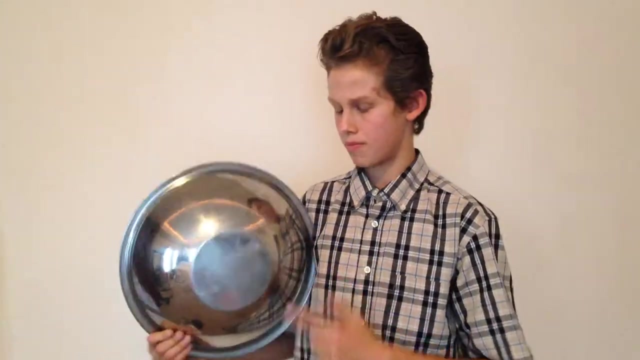 No way. So what is it about a rounded bottom? So when it's on the bowl on the stove, It's sitting there, The stove is really hot, It transfers heat into the bottom, It transfers heat into the middle, causing it to blow out. 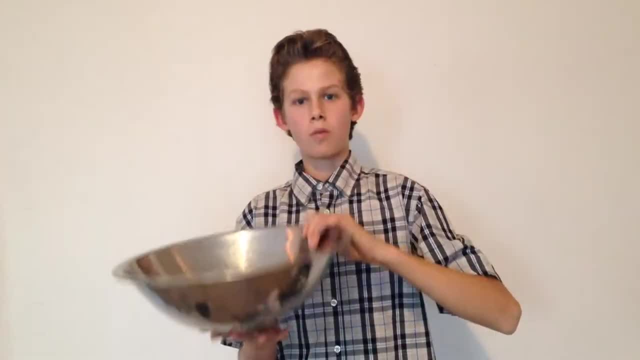 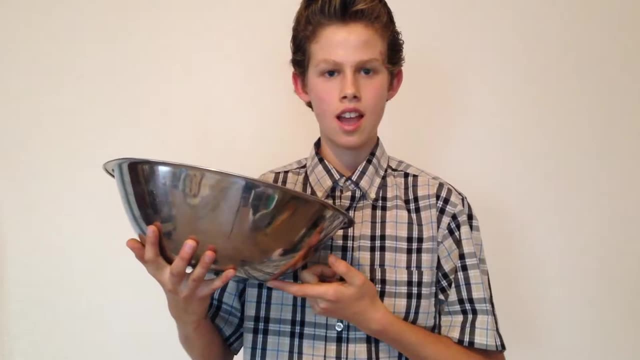 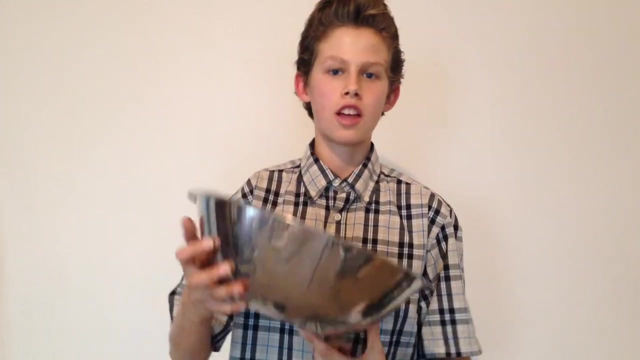 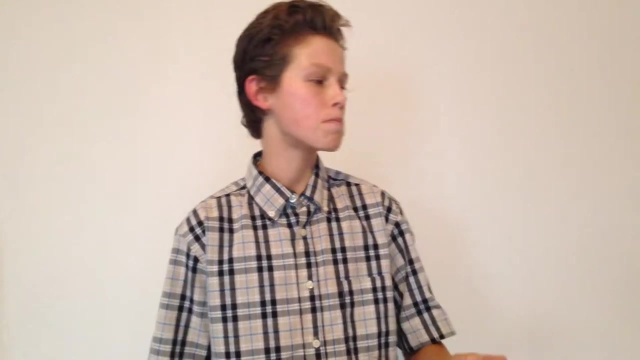 Shifting the center of gravity upwards. It wants to tip over to one side, then it heats the side that it tips over onto, Then it flips back over the other direction, Heats this up and then flips over the other direction. The water inside of it allows it to cool down or whatever liquid you're doing soup. 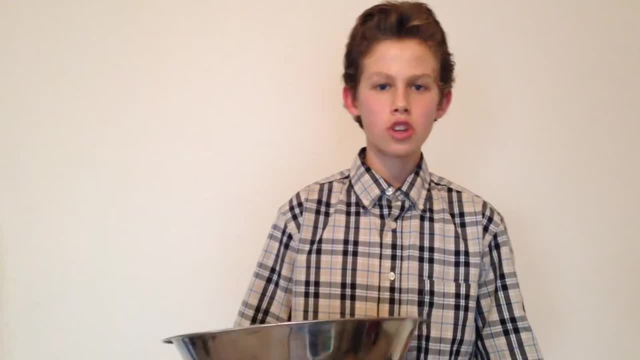 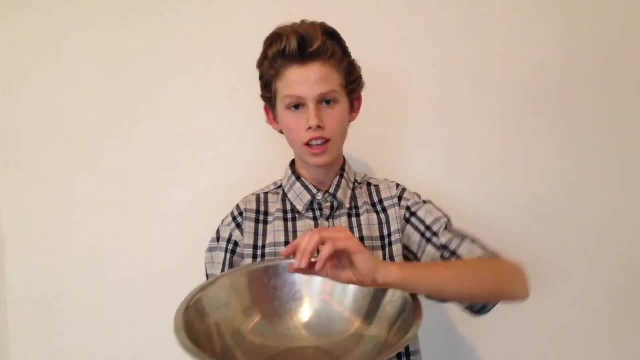 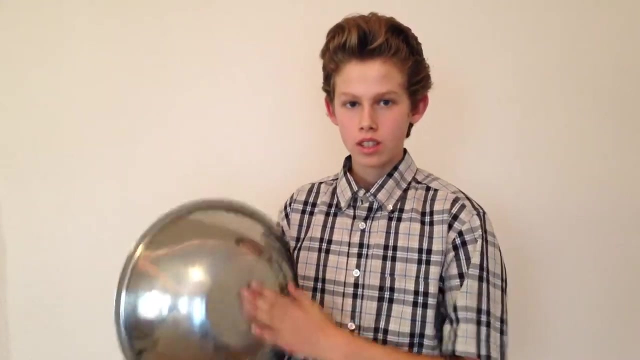 a breakfast cereal. anything you're trying to warm up, it'll do that too with one of these stainless steel bowls. This is really cool. Another reason why you saw so many of those little ripples on it is because when I stuck this bowl on there, the bottom was wet. 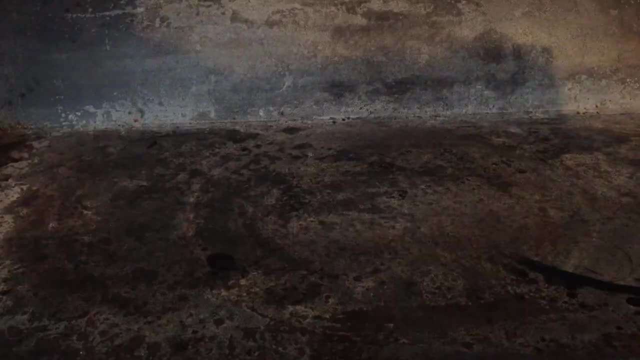 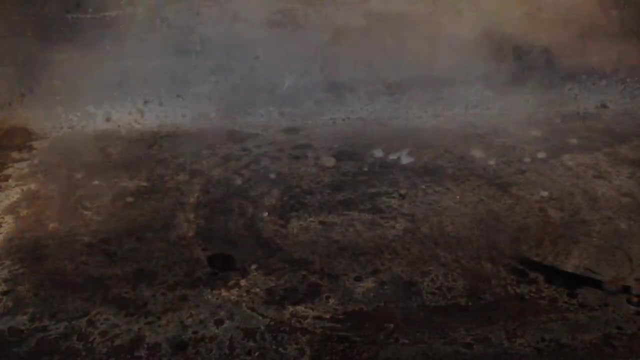 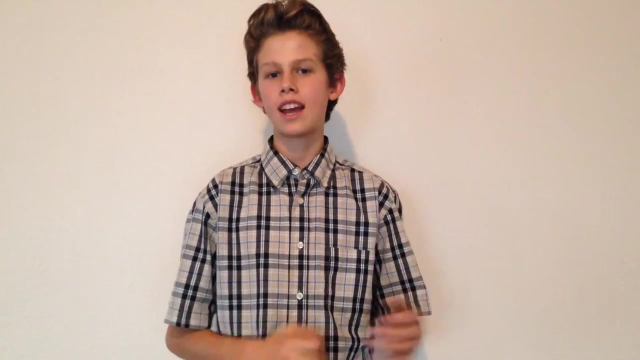 Water. when it comes in contact with something very hot, It instantly turns into steam. so it turns into steam, creating a little explosion because steam has nowhere to go, allowing to have those extremely loud and nice popping sounds. Thank you for watching. If you have any ideas that you would want me to try, please put them in the comments.